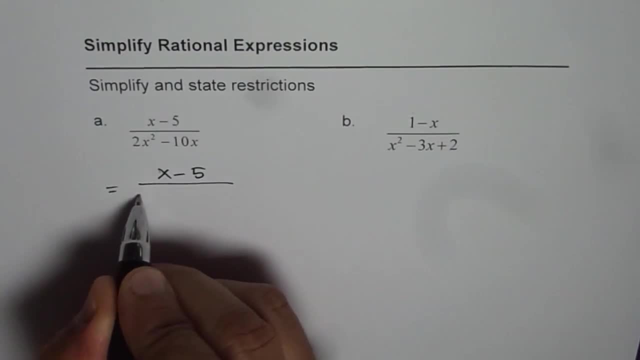 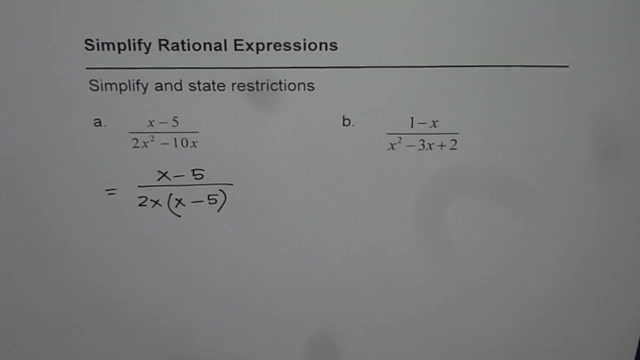 We can write this expression as x minus 5 divided by 2x. Now, when you divide 2x squared by 2x, you get x. When you divide 10x by 2x, you get 5.. So we have x minus 5.. Now, as you can see, when we simplify, x minus 5 and x minus 5 are common factors. They cancel out, and so we can write our simplified expression as 1 over 2x. 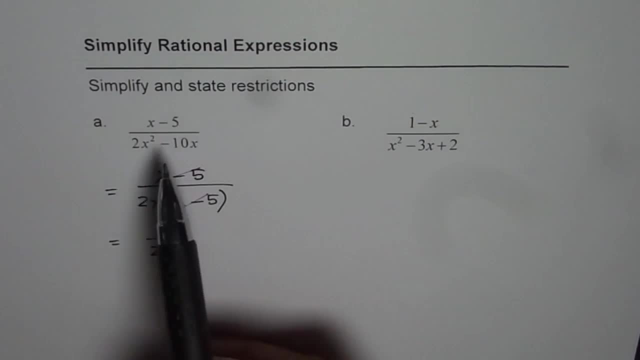 Now the question is: is the expression x minus 5 divided by 2x, squared minus 10x, equal to 1 over 2x? Think about it Well. here the restriction is that x is not equal to 0.. How about this expression In this or that? the restriction is that x is not equal to 5. also, x not equal to 0 and x not equal to 5.. 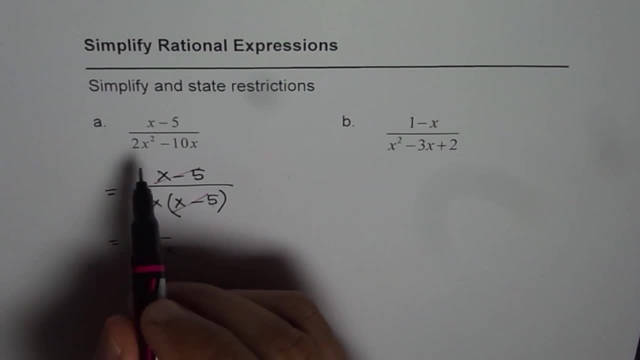 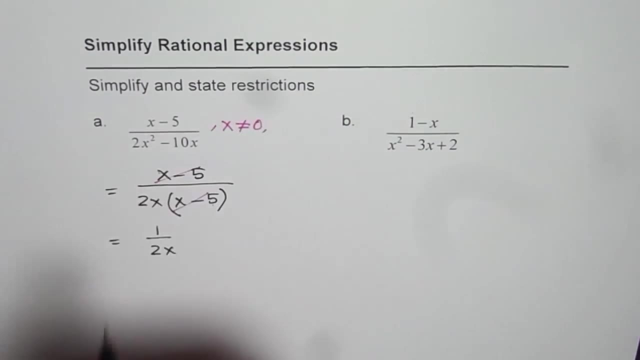 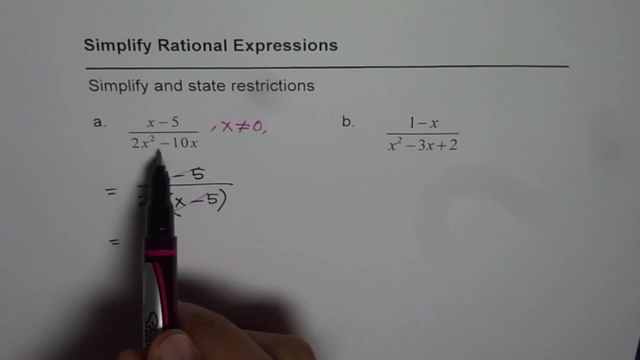 In fact in the original expression, if I write x as 0, you'll get 0 in the denominator, and that is a restriction. So we say: x is not equal to 0.. Second, if I write x as 5, 5 squared is 25,, 25 times 2 is 50 minus 10 times 5 is 50, also gives you 0 in the denominator. So the expression has two restrictions. One: x is not equal to 0.. The other one is: x is not equal to 0.. 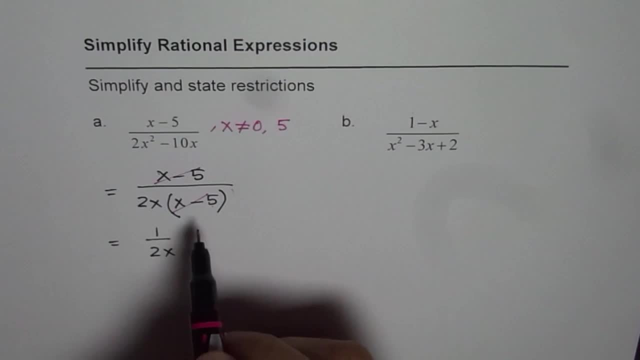 Now, that is a good reminder. So when you are simplifying, at the time when you cancel out the terms, you have to add the restriction here. right, You should say x is not equal to 5 as soon as you cancel out a term, So that at the end you know it is 1 over 2x where x is not equal to 5.. 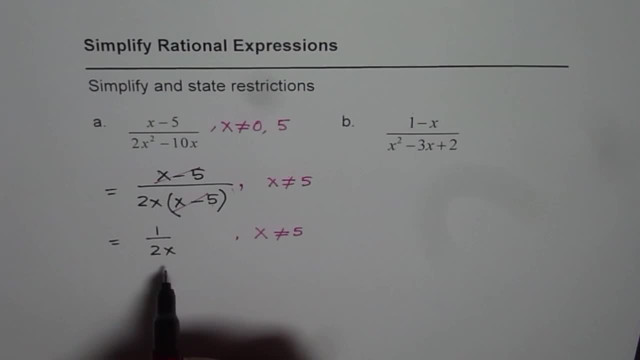 Now, when you look at this simplified expression, we have another restriction, which is x is not equal to 0 also. So the function or the expression which you are working with has two restrictions. You should always write these restrictions before cancelling out. That's the whole idea. 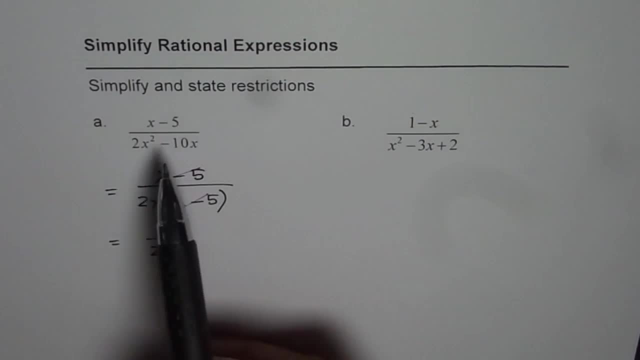 Now the question is: is the expression x minus 5 divided by 2x, squared minus 10x, equal to 1 over 2x? Think about it Well. here the restriction is that x is not equal to 0.. How about this expression In this or that? the restriction is that x is not equal to 5. also, x not equal to 0 and x not equal to 5.. 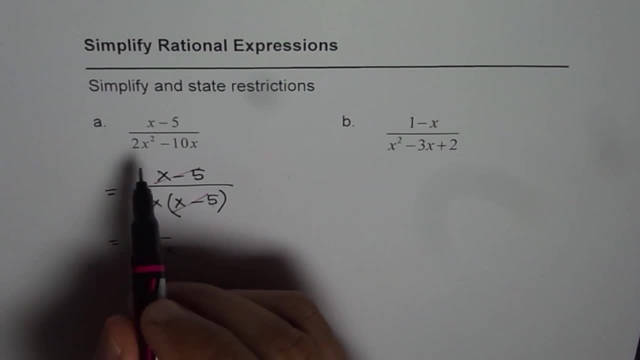 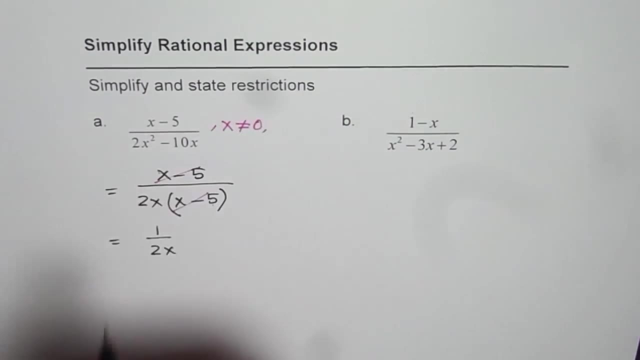 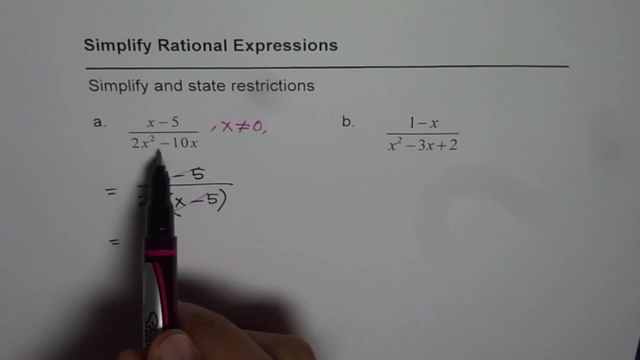 In fact in the original expression, if I write x as 0, you'll get 0 in the denominator, and that is a restriction. So we say: x is not equal to 0.. Second, if I write x as 5, 5 squared is 25,, 25 times 2 is 50 minus 10 times 5 is 50, also gives you 0 in the denominator. So the expression has two restrictions. One: x is not equal to 0.. The other one is: x is not equal to 0.. 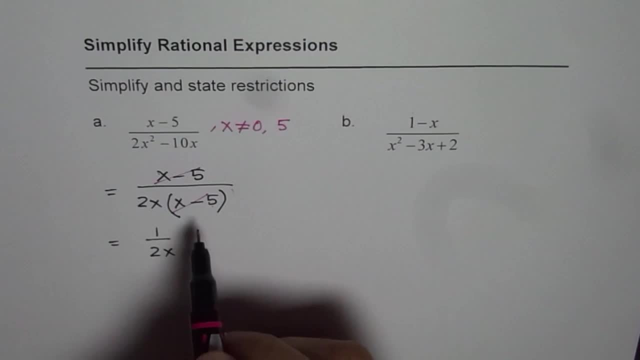 Now, that is a good reminder. So when you are simplifying, at the time when you cancel out the terms, you have to add the restriction here. right, You should say x is not equal to 5 as soon as you cancel out a term, So that at the end you know it is 1 over 2x where x is not equal to 5.. 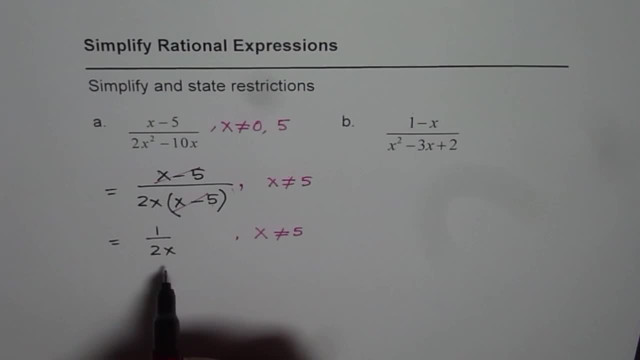 Now, when you look at this simplified expression, we have another restriction, which is x is not equal to 0 also. So the function or the expression which you are working with has two restrictions. You should always write these restrictions before cancelling out. That's the whole idea. 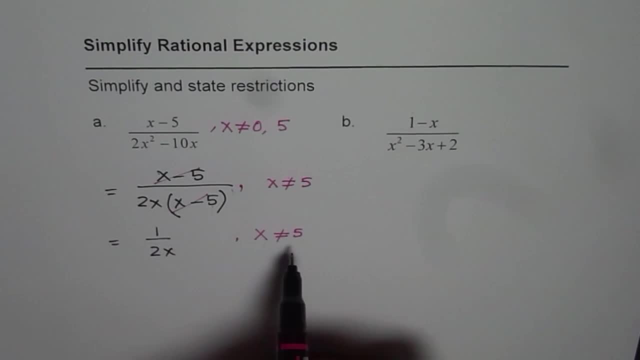 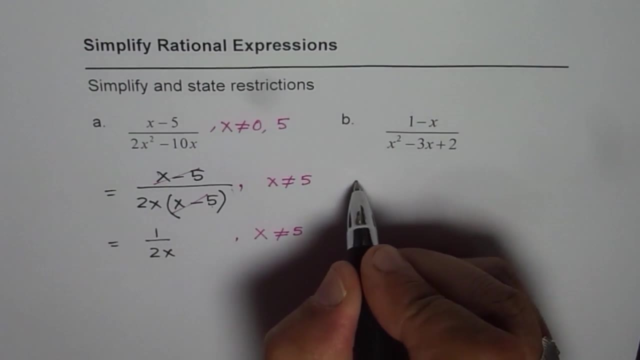 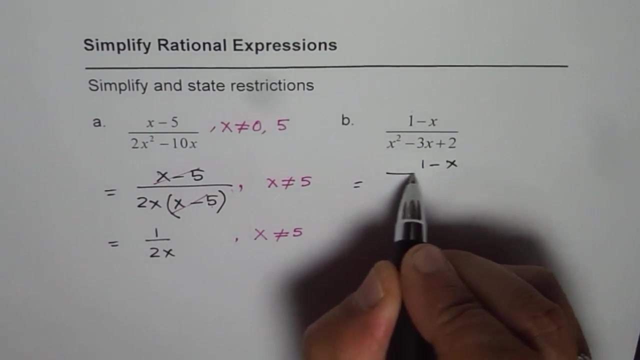 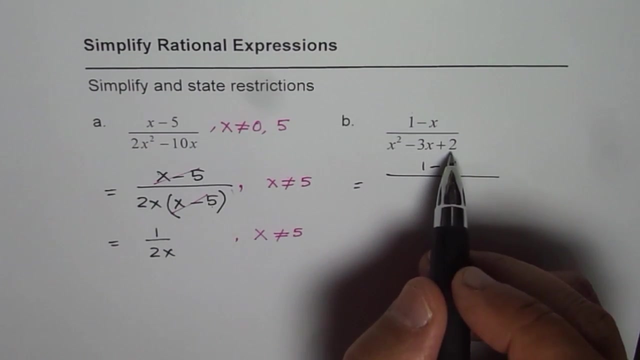 So remember that part. So don't forget to include 5 amongst the restrictions. So let's do the next one Now. to simplify, as I said, is to find common factors right. So 1 minus x In the numerator, here we have x squared minus 3x plus 2.. We can factorize: 2 times 1 is 2.. We need minus 3 as a sum, So it should be minus 2 times minus 1..